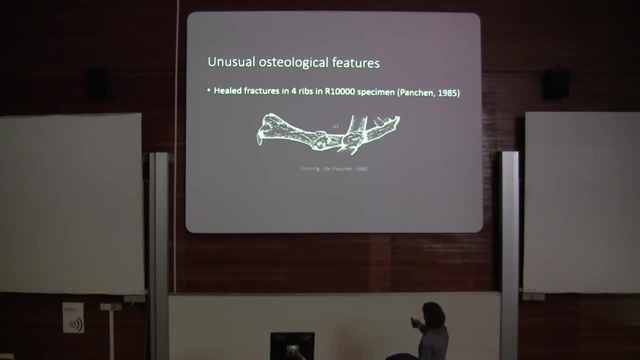 see by the ankylosed bone here and here, And they also found an unusual morphology in the distal femur and the proximal tibia and it's on both sides, So the femur is the left and the tibia is the right And this is unique to Crassidarium and it was initially interpreted. 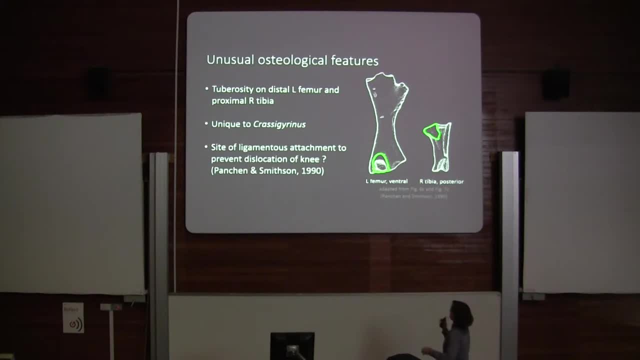 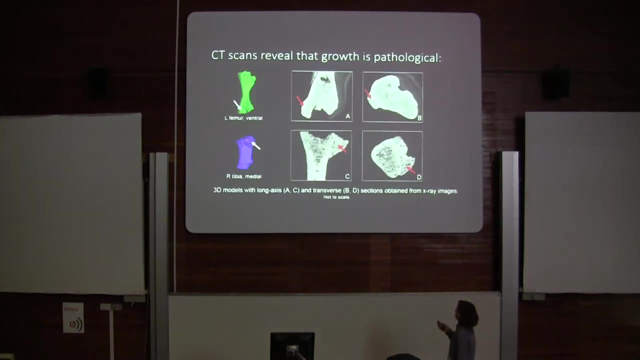 as being a function And it's a very unusual feature due to maybe there was a ligamentous attachment if this animal was using its back limbs to paddle in the water to prevent dislocation. But I took CT scans of these specimens and it becomes apparent that this is a pathological. 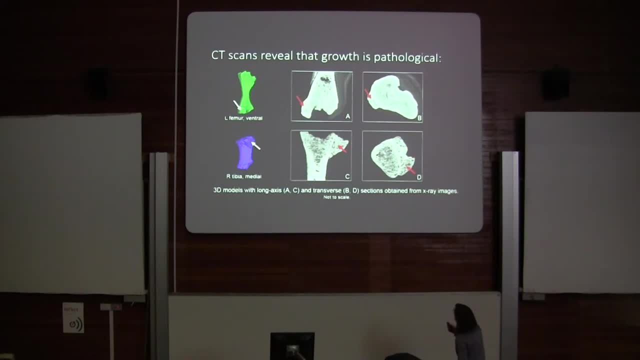 feature. So these scans are a little hard to see. but you can see the cortical bone here, the denser white, and then this is the trabecular bone And then this growth looks very much separate. so it's probably secondarily depositing bone here And you can see there's. 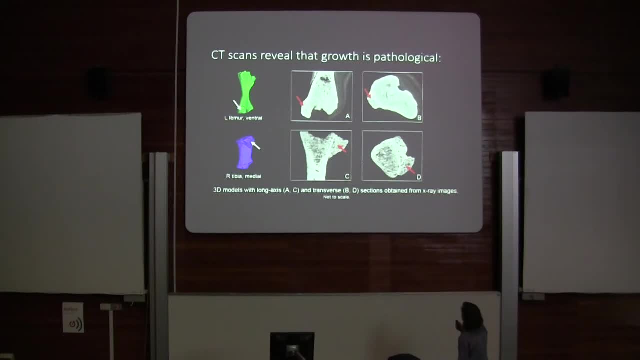 some cortical bone here. Same view, but transverse section right here- And then this is in the tibia: a very similar thing. So this is what it looks like on the actual bone, And so this led me to conclude that it's either due to some sort of single traumatic event. 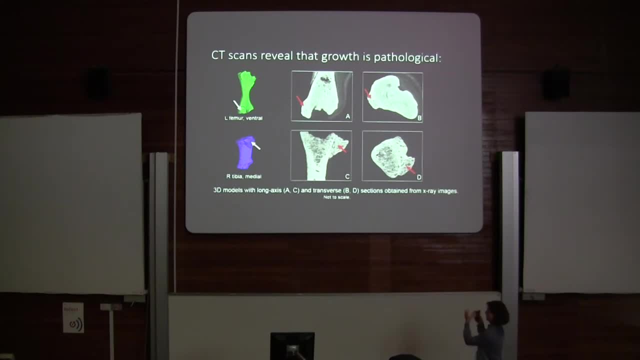 So maybe we don't see a fracture line, which is unusual, and it's only found on one side of all these bones, which is also unusual, But the fact that the cortical bone is so distinct makes it look like it's some sort of pathology that's either related to a single 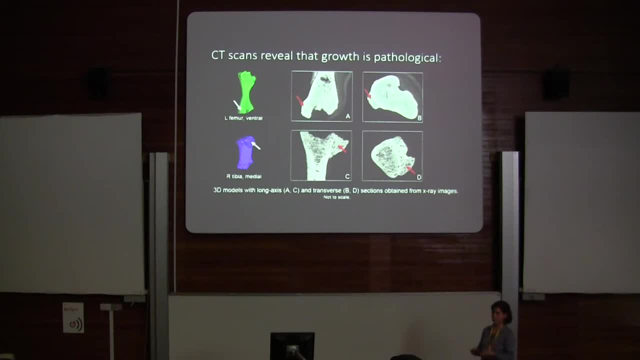 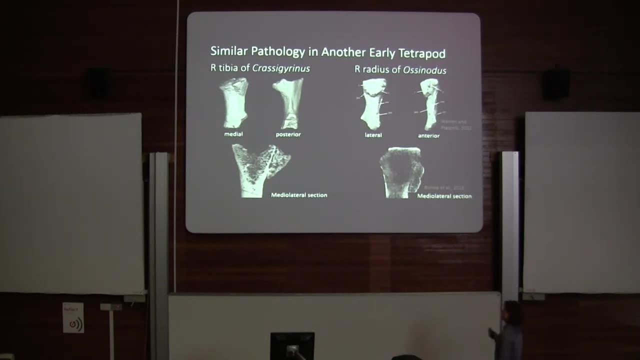 trauma or maybe repeated stress, so more like osteophytosis where the bone is remodeling to compensate for that stress. So I looked at other early tetrapod literature and I found a very striking similarity in the proximal radius of Ossinotus. Ossinotus is also an early tetrapod, about 2 million. 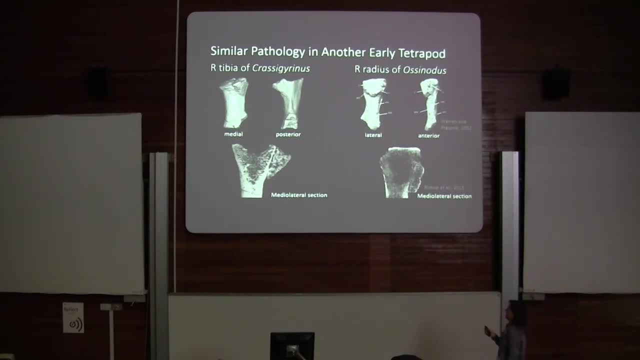 years older than – sorry, 10 million years older than Crassogyrinus, but similar depositional context And a paper used this pathology on Ossinotus to claim terrestriality in this animal and I found that this pathology is very similar to the pathology of Ossinotus And I found that this pathology is very similar to the pathology of Ossinotus, and I found that this pathology is very similar to the pathology of Ossinotus. and I found that this pathology is certainly comparable because they said this fracture must have happened during a fall. 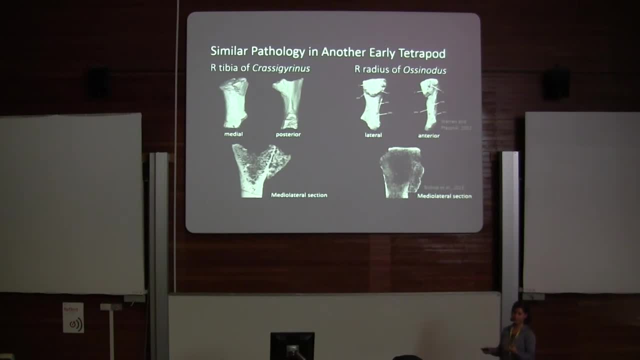 on land, because only that loading environment could have caused that injury and the subsequent bone remodeling. but since we see this as a very similar injury – and you can see A very similar injury, and you can see that both in the cross-sections and the models.